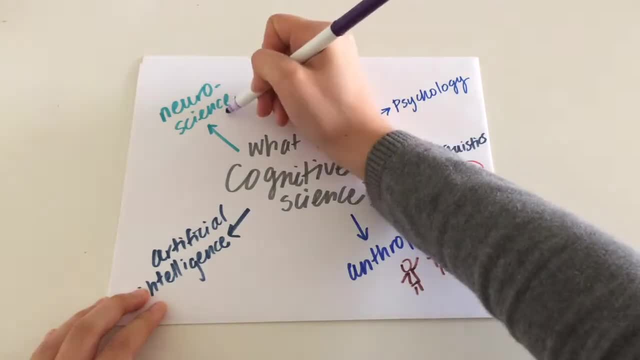 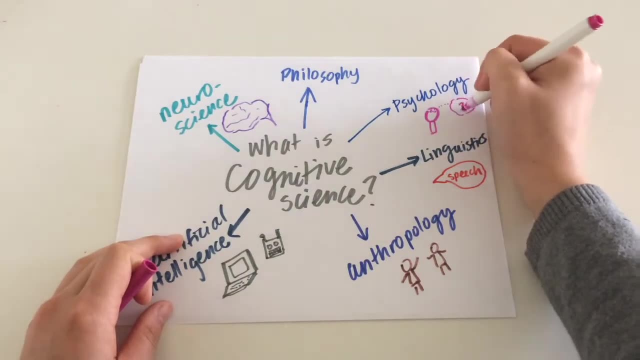 questions about the mind, like: how does culture and shared knowledge influence the way people interact with and perceive the world around them? What are ways that we could teach machines to mimic the way humans process information? How does language learning come so naturally to infants? 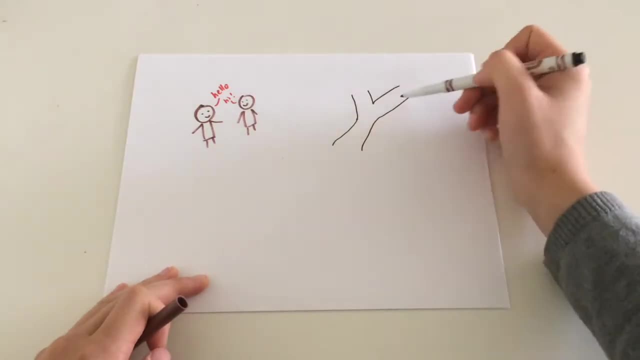 Or when life presents us with two paths we could go down. it's amazing that we're able to pull from our past experiences, as well as predict future events, to make an informed decision, Or that we could visualize numbers in the form of graphs and equations. We are able to perceive the 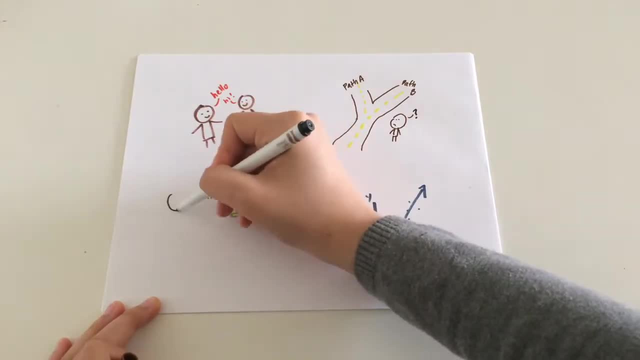 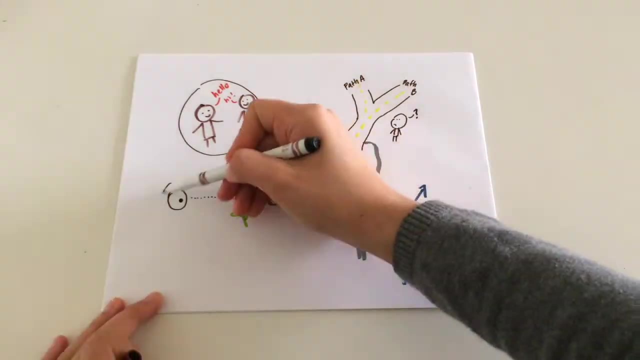 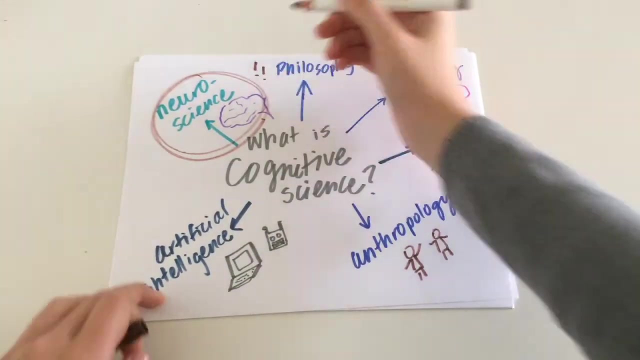 flower in front of our eyes and admire its color, texture and inherent beauty. These high-level processes all link back to some network in our brains. Neuroscience aims to decode and uncover the mysteries behind the underlying hardware that makes all of this possible. Neuroscience is the study of the nervous system, which largely involves the brain. 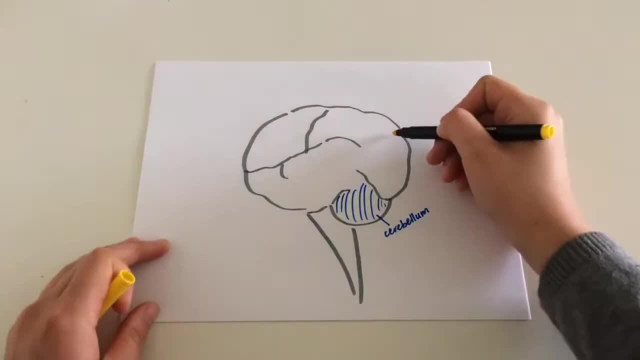 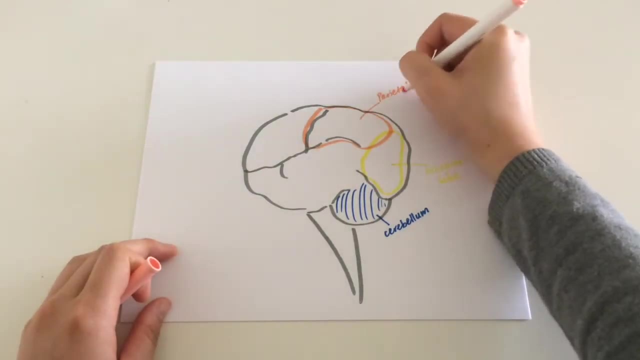 Understanding the brain's anatomical structure is crucial towards mapping out the functions of each part. It allows us to get a better picture of how neurons wire together to form an incredibly complex network and how these neural circuits give rise to a more complex network- Neuroscience- 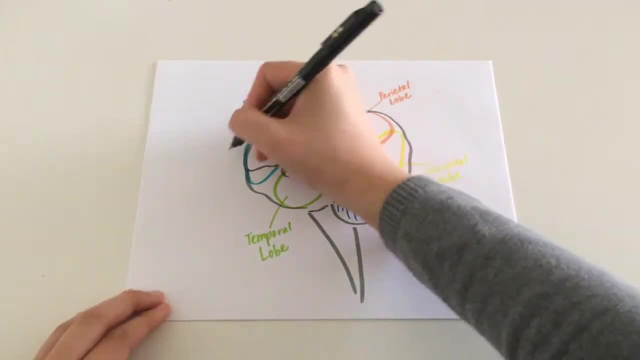 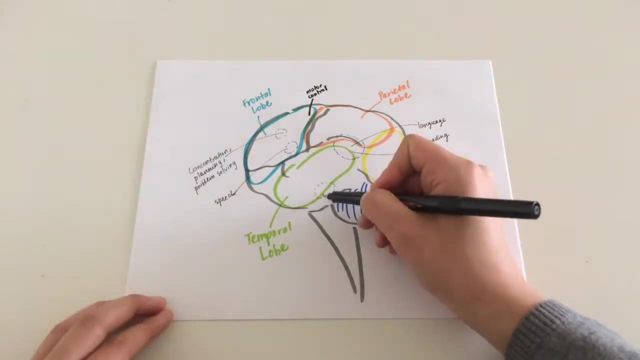 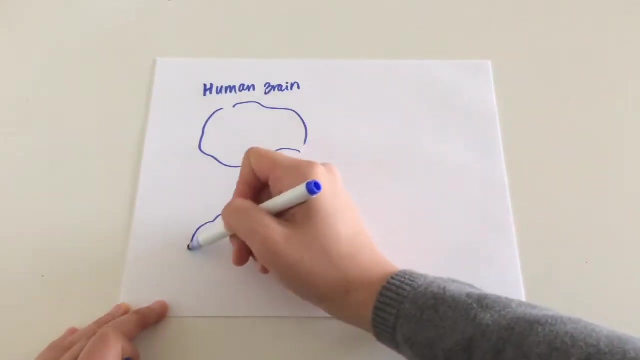 gives rise to those high-level processes that humans can perform. What distinguishes neuroscience from other disciplines, and how could cognitive science borrow from its research methods? Neuroscience tends to take a more biological approach to studying the brain in order to answer questions concerning the physical mechanisms behind behavior. 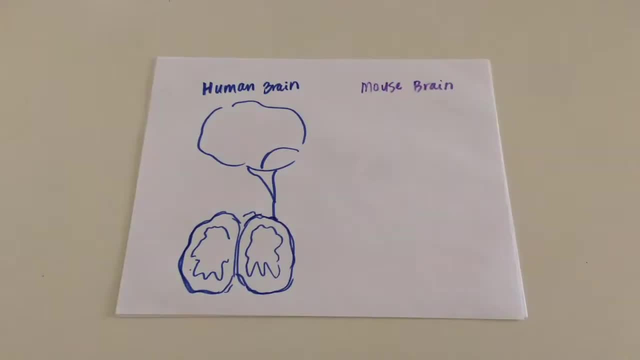 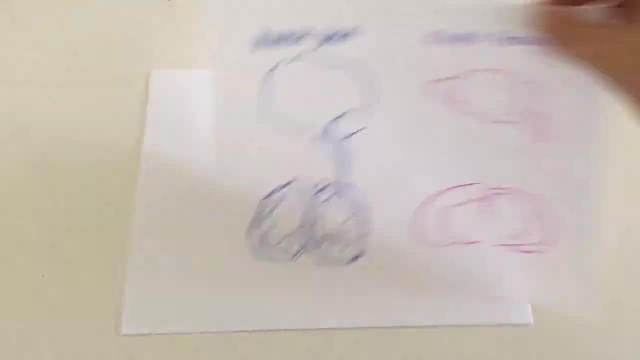 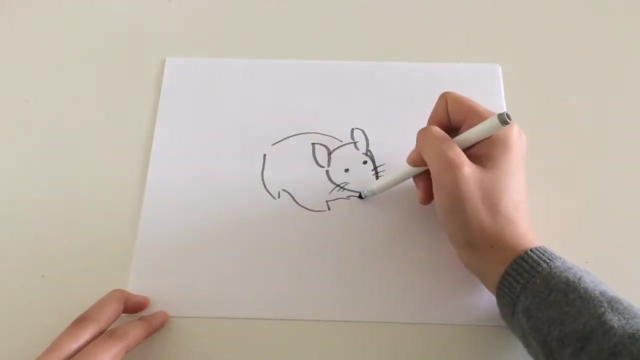 Neuroscience research tends to use animals like mice to study the brain's anatomy and physiology, since it turned out that mice brains share quite a few similarities with human brains. Neuroscientists also probe directly into mice brains to stimulate or observe the firing rates of certain regions as they perform tasks like navigating physical space or learning an. 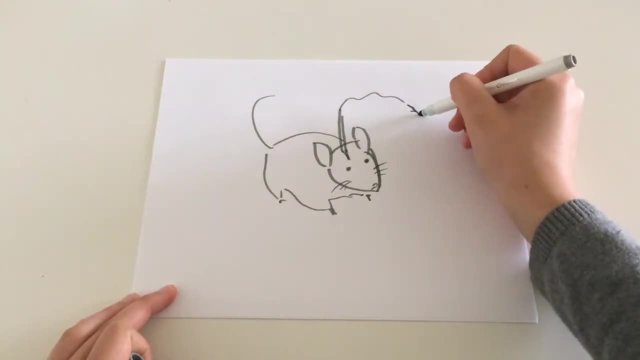 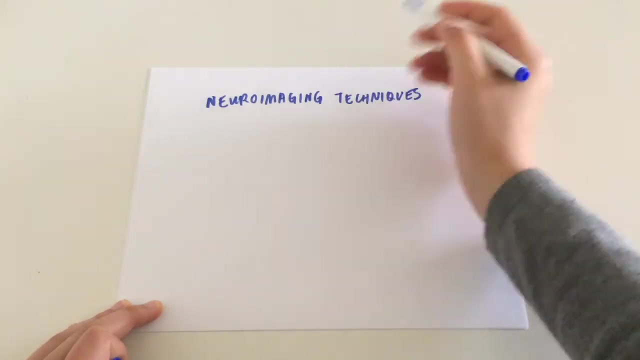 association. This way, we could directly view and track neural activity. Scientists also delete gene sequences to create knockout mice in order to observe the effects of inactive brain areas. We could also observe neural activity with human subjects using neuroimaging techniques. Each have their own pros and cons, but in any case, it's amazing that these technologies